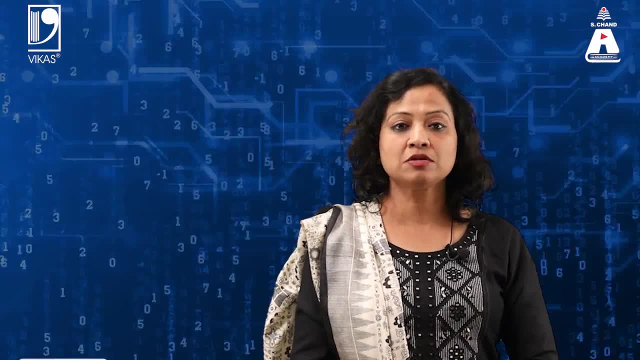 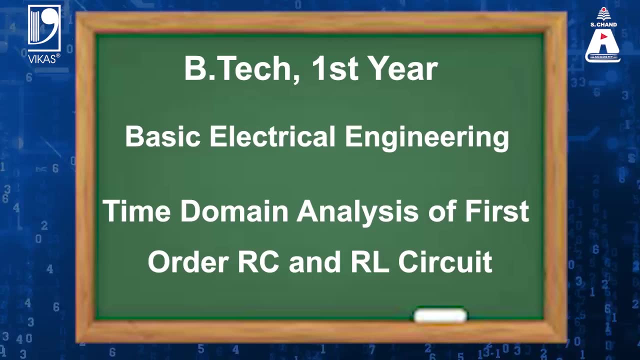 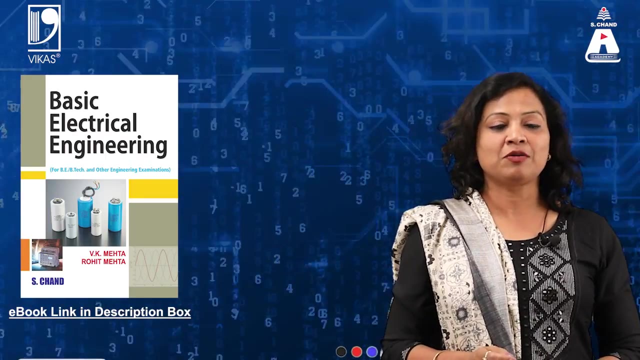 we will discuss about this. transient response or time domain response of RC and RL circuit. Hi, I am Professor Anjali Gaur and welcome to S Chand Academy. To know more about this topic, you can refer to this book by S Chand Publishing, the link to which is given in the description box. 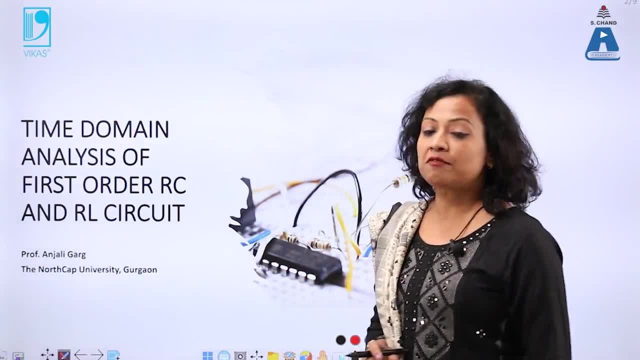 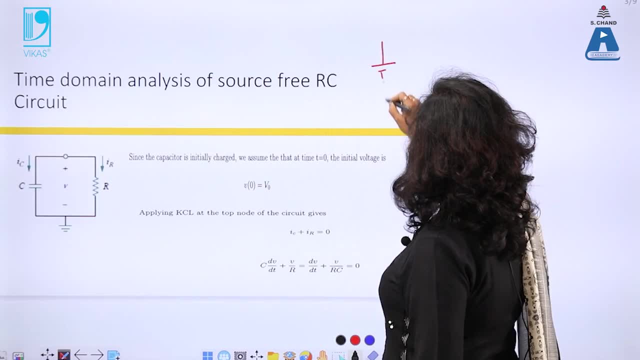 below. Today we are going to discuss about the RC and RL circuit. Time domain: analysis of first order RC and RL circuit. So I have a circuit like this. Suppose I have a circuit like this and there is a switch. There is a switch which consists of: 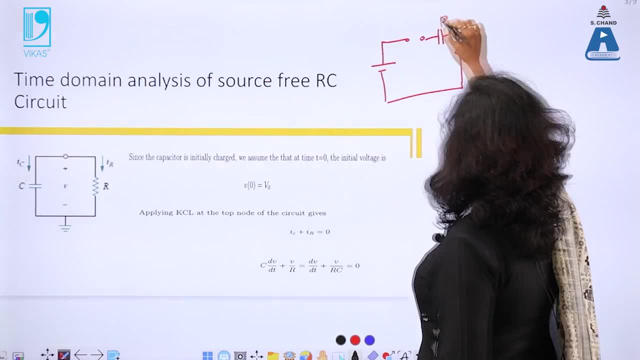 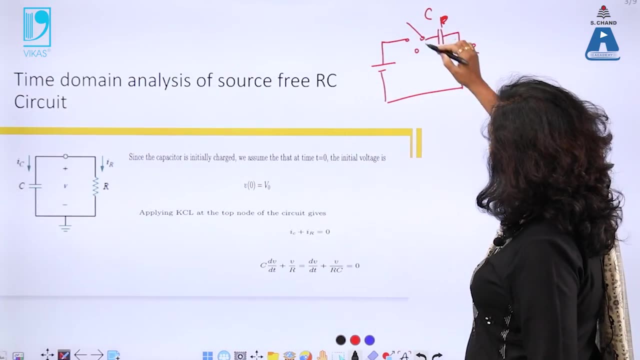 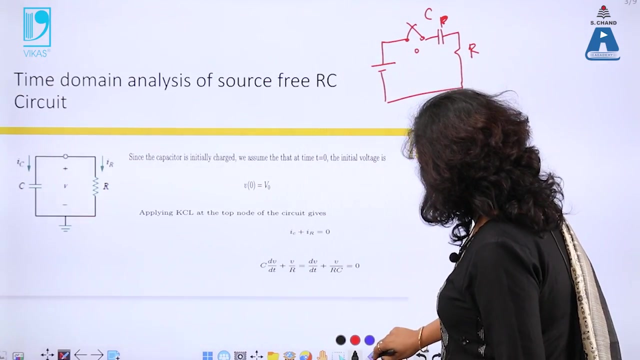 the circuit consists of R and C. This is my C and this is my R. So initially- and there is one more point- So this switch is initially closed at this point and my capacitor is fully charged now and after certain instant, after certain instant, I connect this to the circuit. 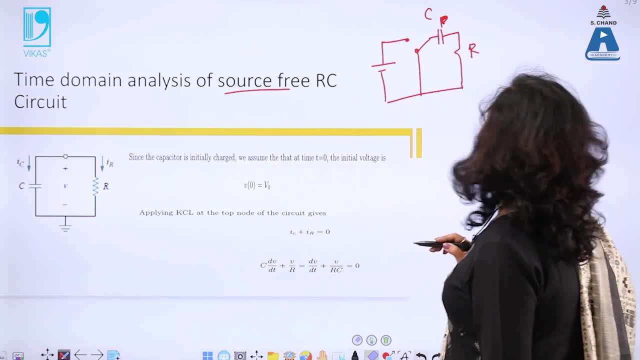 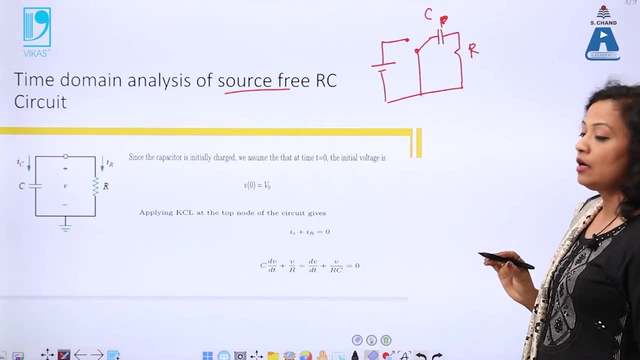 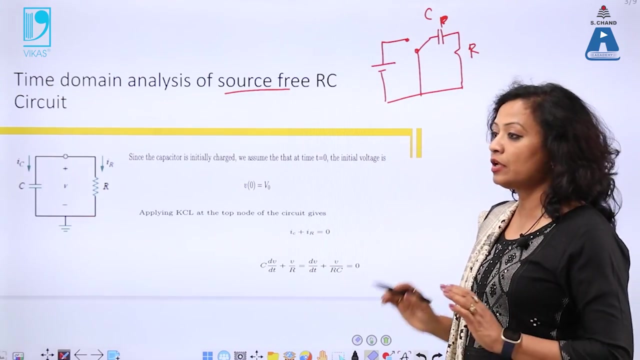 like this now this is called as source free RC circuit, where the capacitor is initially charged and now discharge within the circuit and finally my current die off, or you can say that my circuit will not have any current after certain instant of time. so initially there is the capacitor is fully charged. 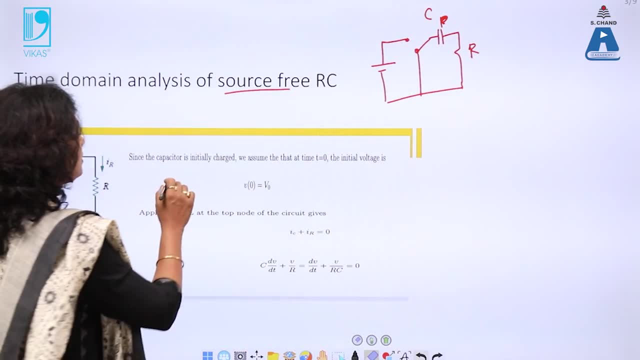 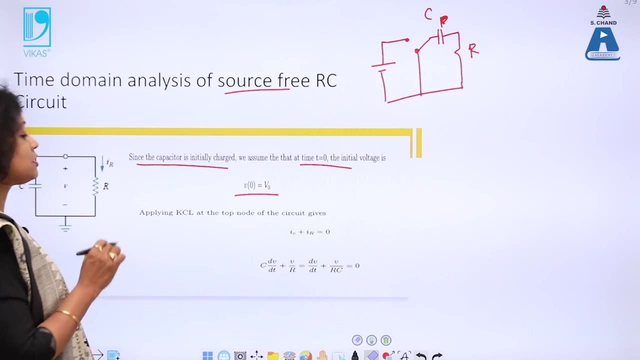 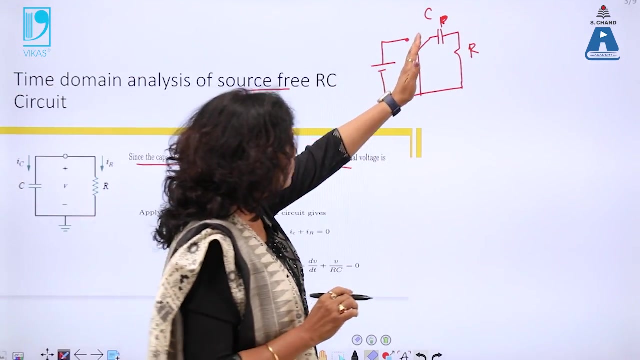 but later on the pastor discharges. since the capacity is initially charged, where zoom that at t is equal to 0, initial voltage is equal to be not which is the maximum voltage or peak voltage of this, and the source free is where the capacitor we have connected this to at this point. so there is no source in the 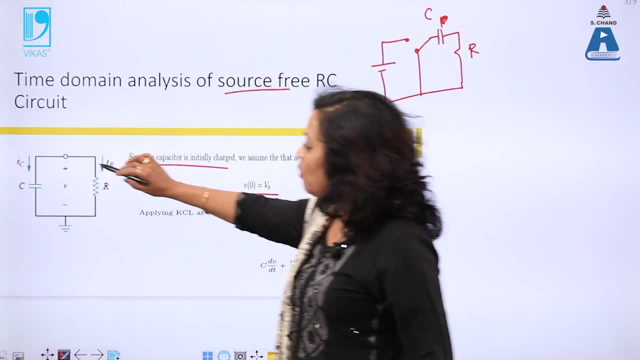 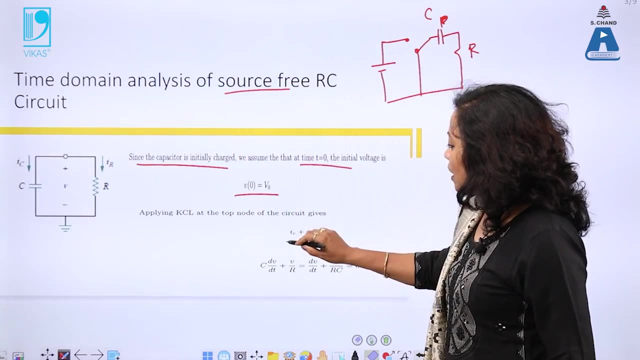 circuit. so my circuit will behave like this: there are two current at this node. I see that is the current and capacitor, I a current and resistance. so you So using KCL. my IC plus IR is equal to 0. So I apply KCL at node. 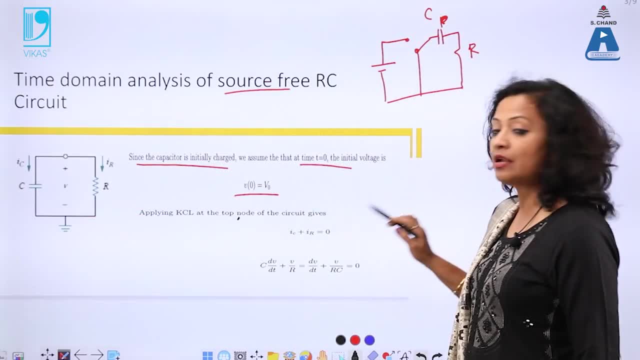 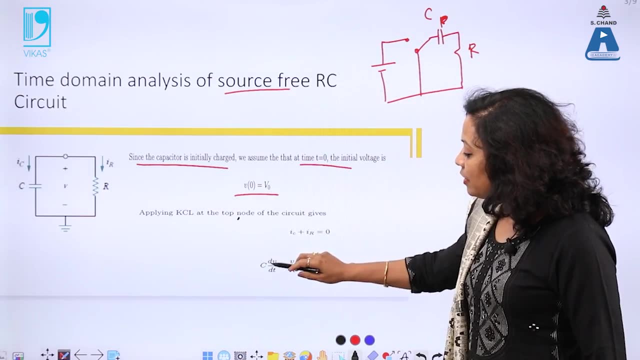 So IC and IR, both are leaving this node. So IC plus IR is equal to 0.. So IC is the current in the capacitor and IR is the current in the resistance. So IC is C dV by dt, as we discussed, in capacitive circuit. 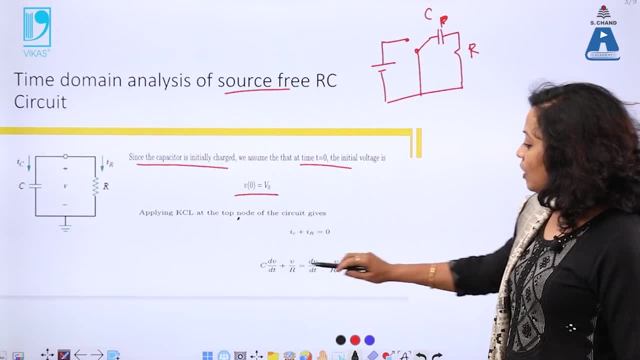 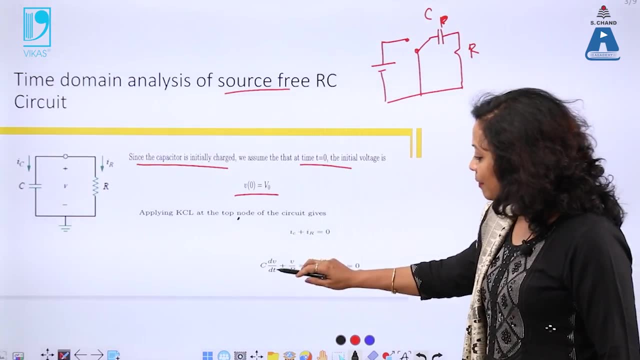 And IR is voltage by resistance, as per Ohm's law. So I have C. dV by dt plus VR is equal to 0.. Now, after reshuffling the elements, dV by dt is I brought C there, So V by RC is equal to 0.. 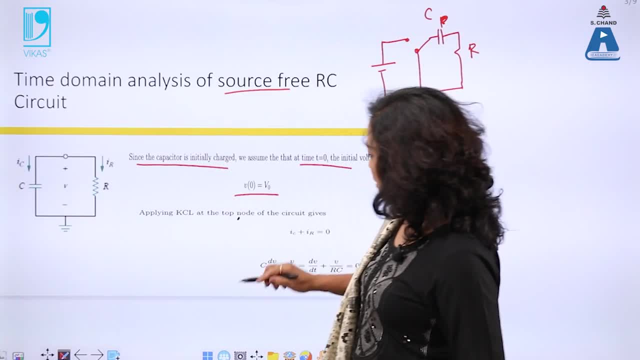 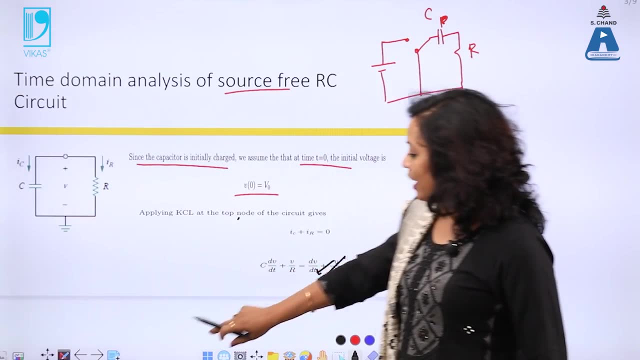 Now let me go back. So I have shifted now this V to this place and this dt to this place, So that I can have dV and V at the same place. So dV by V is equal. So dV by V is equal to minus dt by RC. 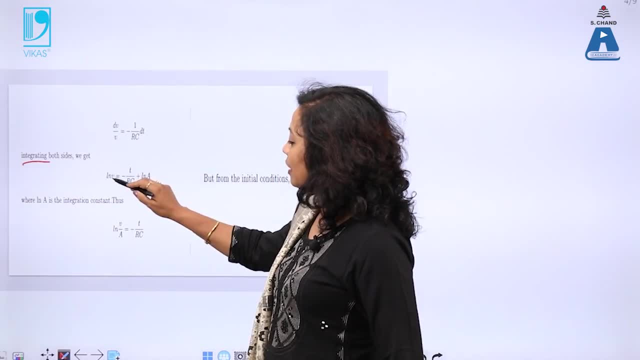 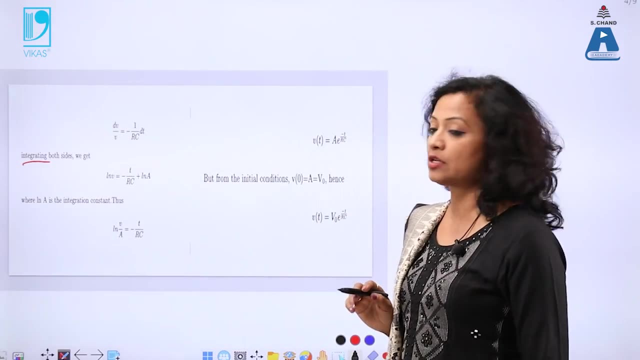 And now integrate both side. So after integrating I am getting ln V is equal to minus t by RC after integration plus ln of A, where ln of A is constant of integration. Now to find the value of ln of A I have to put the initial condition. 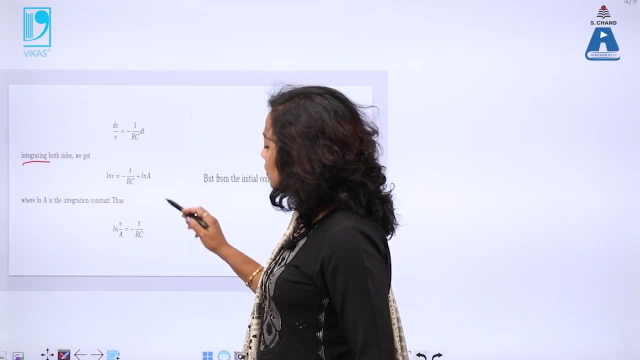 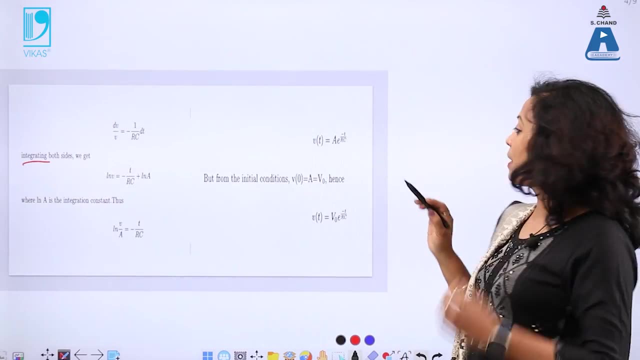 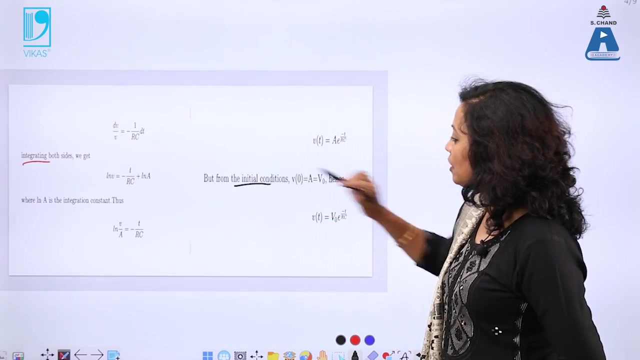 So ln of V by A is equal to minus t by RC, And if I solve this I will get Vt is equal to A. So ln of A is equal to minus t by RC, where A is integration constant. And to find the value of this A I put initial condition. 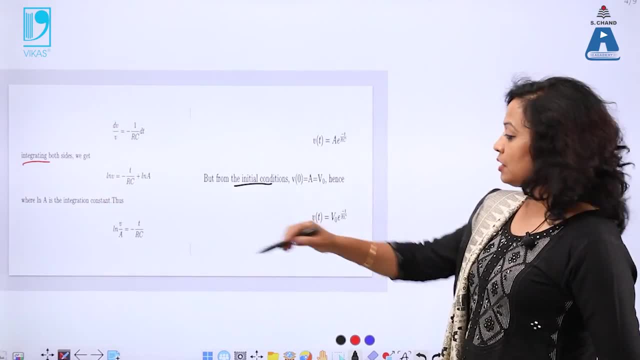 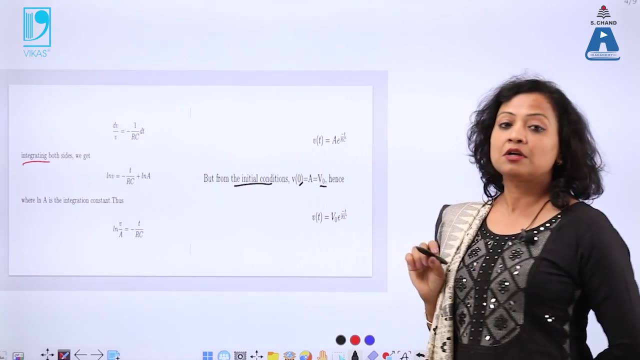 So what is initial condition? We discuss just we discuss that initially capacitor is fully charged. So initially, when t is equal to 0, my voltage is full voltage. That is, capacitor is fully charged And whole input voltage appears across the capacitor. 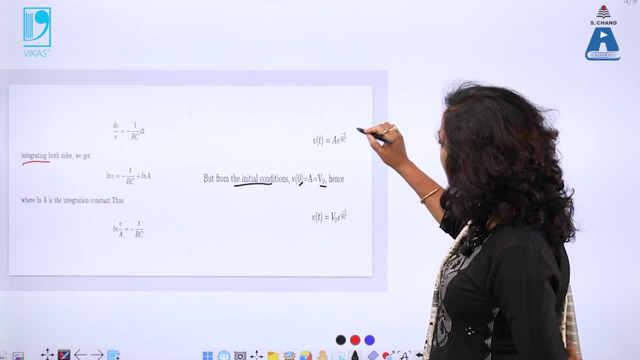 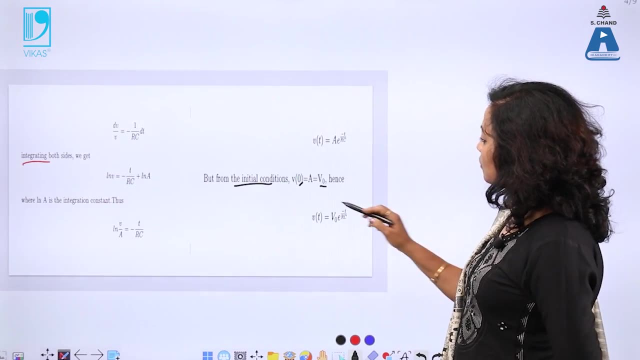 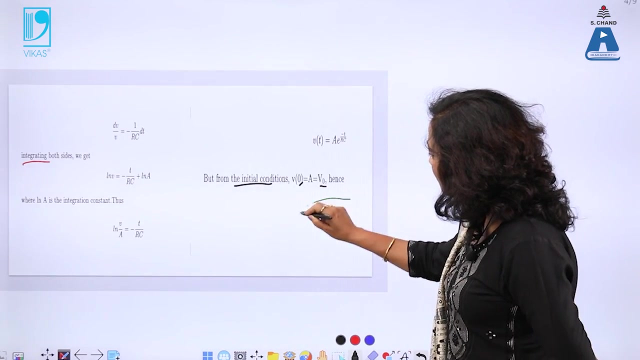 So at t is equal to 0,. if I put t is equal to, if I put t is equal to 0, I get V0 is equal to A. V0 is equal to A. So my A is V0.. So this is my, this is my equation of voltage at time: t, which is equal to V0. 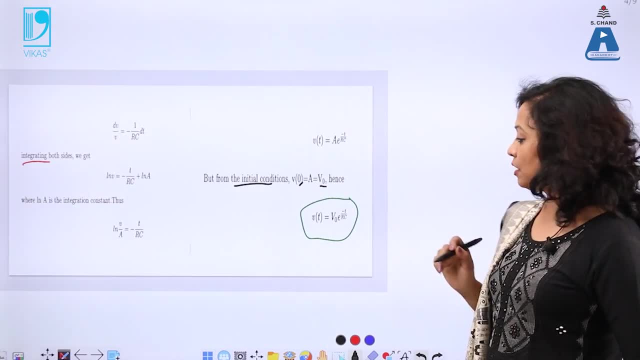 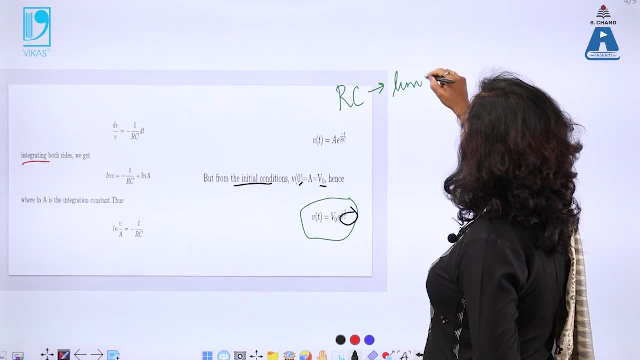 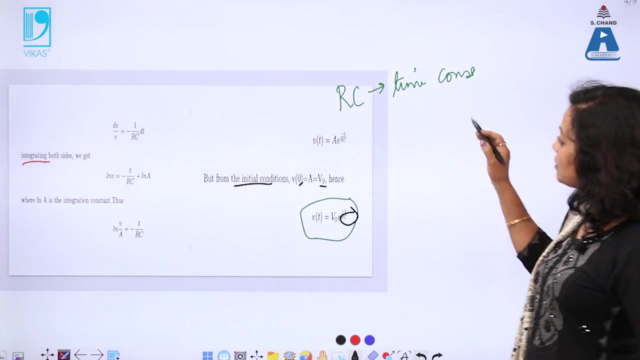 That is a peak value of voltage, e power minus t by RC. Now this RC, this RC is called as time constant, Which depends upon elements which we choose in the circuit. So, based on the value of R and C, my time constant varies. 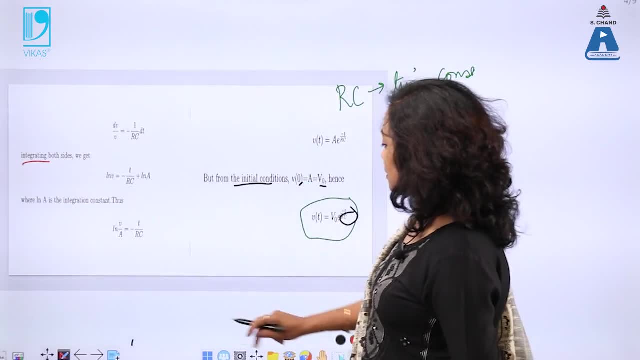 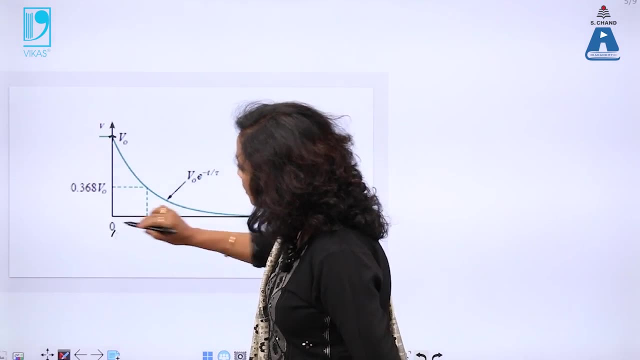 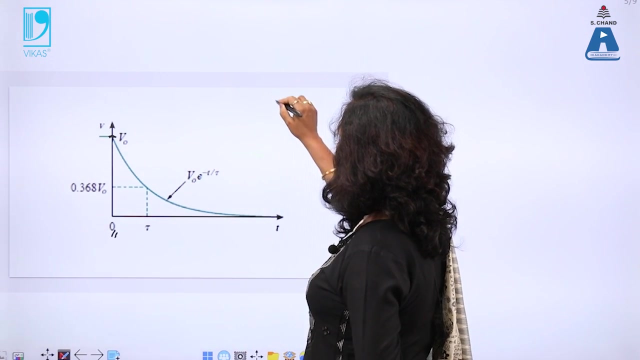 And that time constant can be shown with this graph. This graph. This graph shows that initially, when t is equal to 0, my voltage is full voltage, That is, peak voltage is equal to V0.. And as the time varies, my Vt. 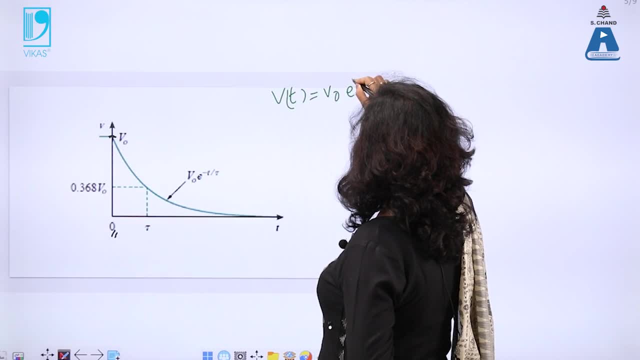 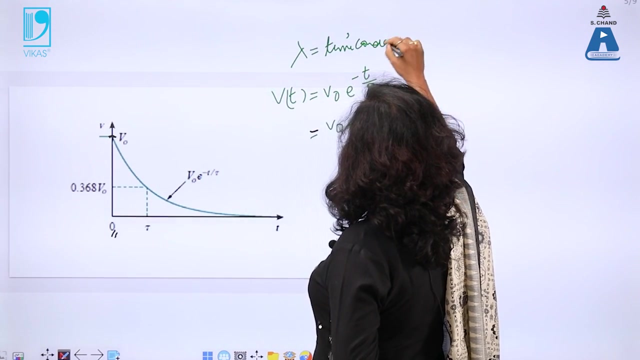 I will write the equation again: V0 e power minus t by RC. Or I can write V0 e power minus t by lambda, Where lambda is time constant And it is given by RC. Now, initially, when t is equal to 0,. 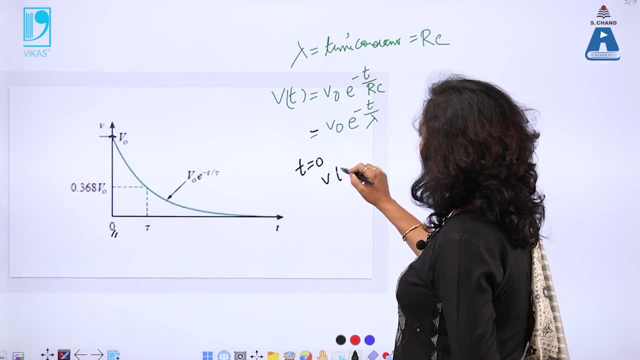 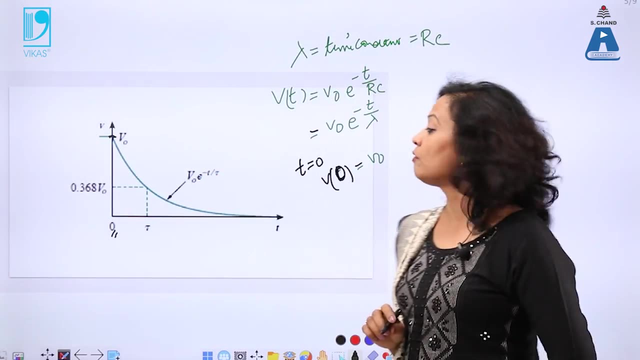 when t is equal to 0, my Vt is equal to V0, rather, V0 is equal to V0. So at t is equal to 0, I am getting maximum value of voltage V0. Now, as the t increases, because this is negative, 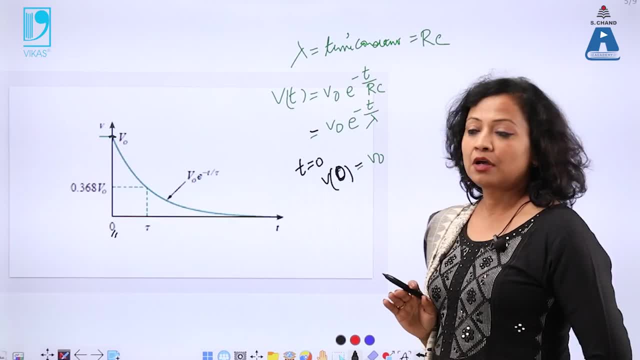 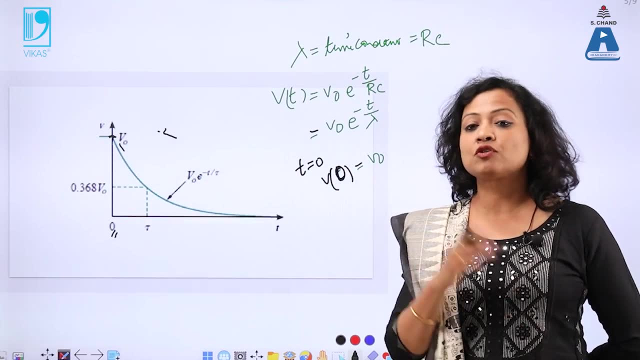 So, as the t increases, this value of voltage goes on decreasing, So this voltage goes on decreasing. And finally, when t is infinite, that means I have switched off, I have removed the source. So after t, infinity time, this voltage will become 0. 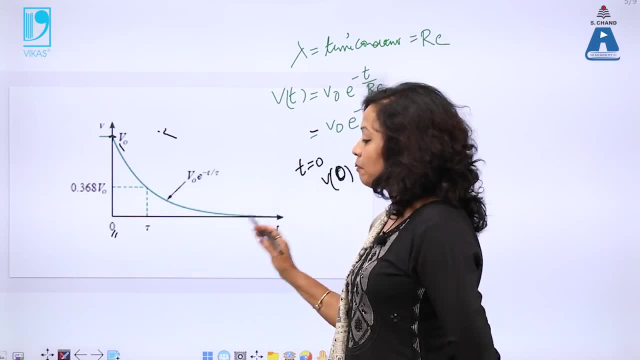 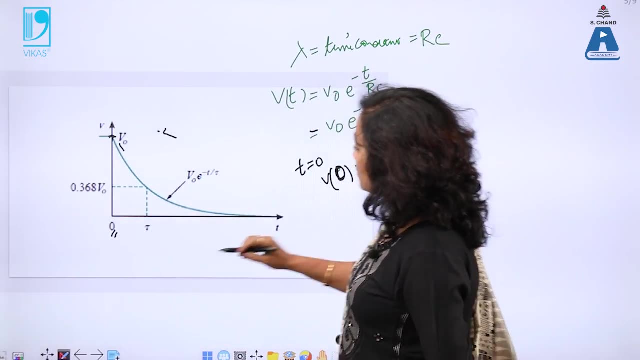 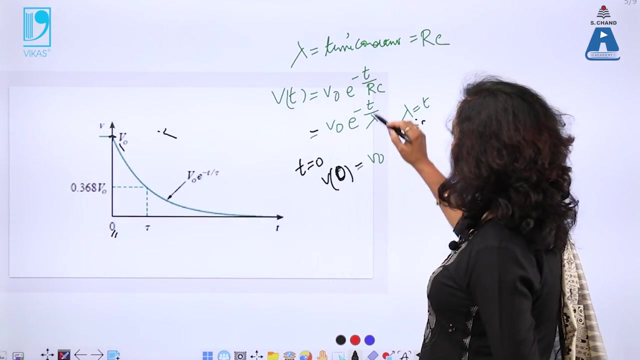 If I put t infinity I am getting V voltage 0. That means capacitor is full, It is fully discharged. Now how to get the value of this time constant. Let lambda is equal to t, So I will put lambda is equal to t. 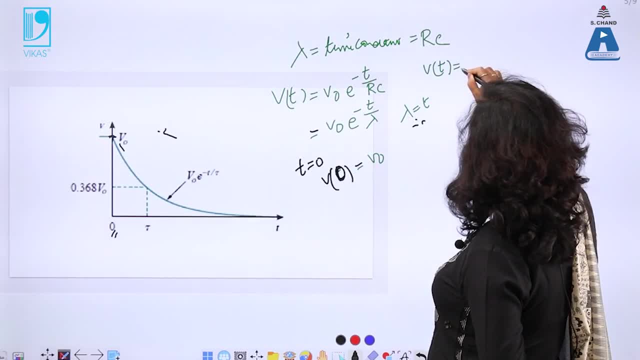 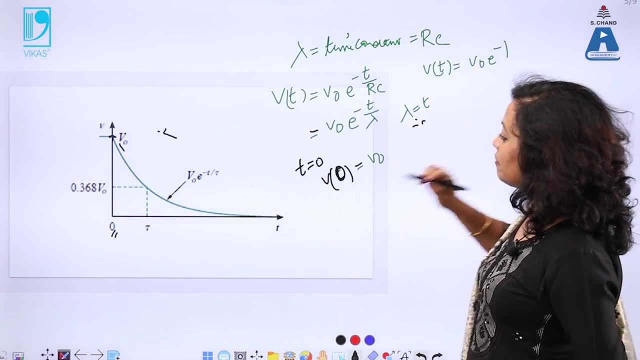 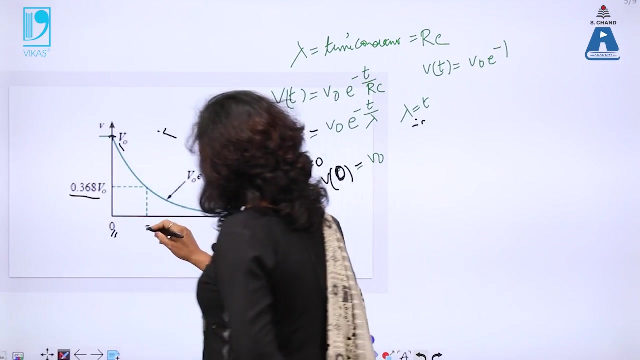 So I will get. Vt is equal to V0, e power minus 1.. So if I put exponential power minus 1, I will get the value 0.368 of V0.. Time constant: this is time constant, This is tau. time constant is that time. 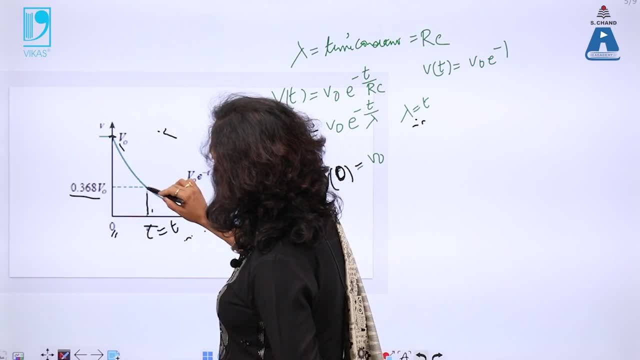 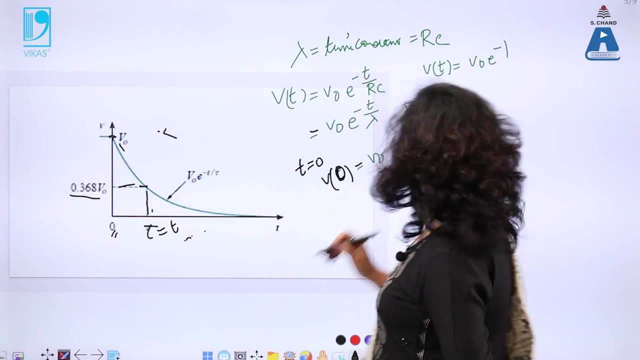 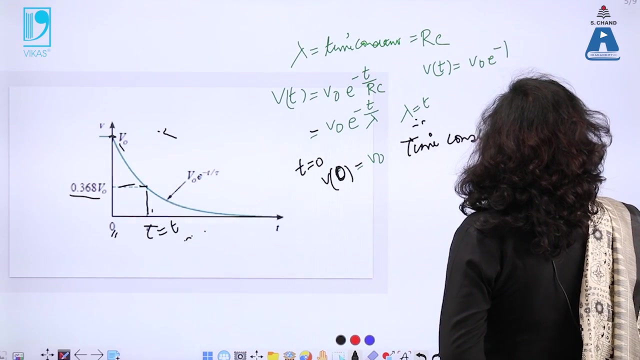 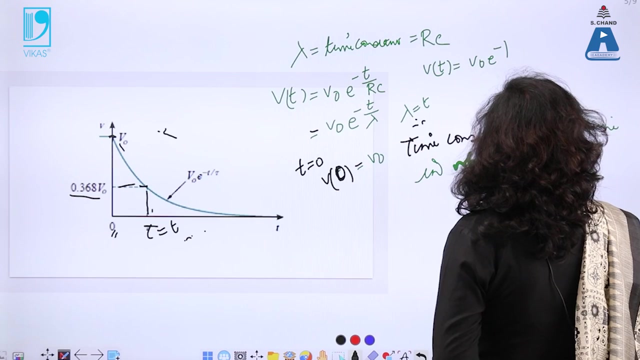 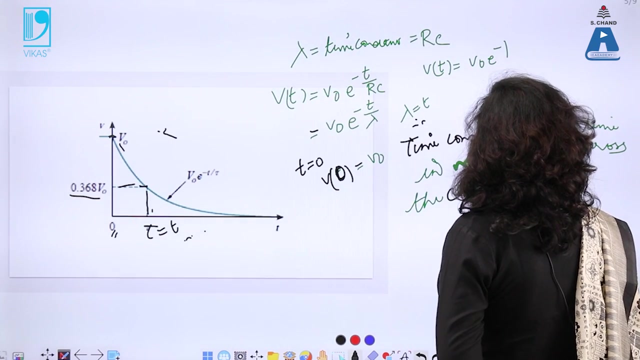 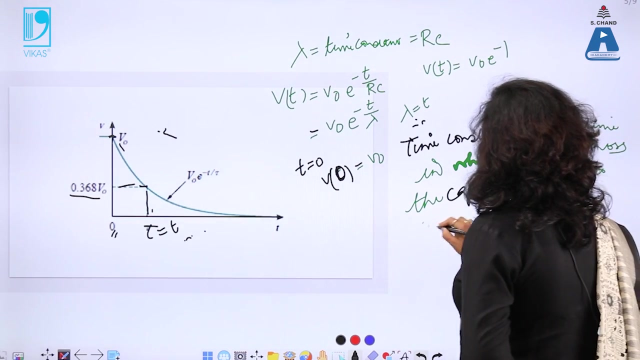 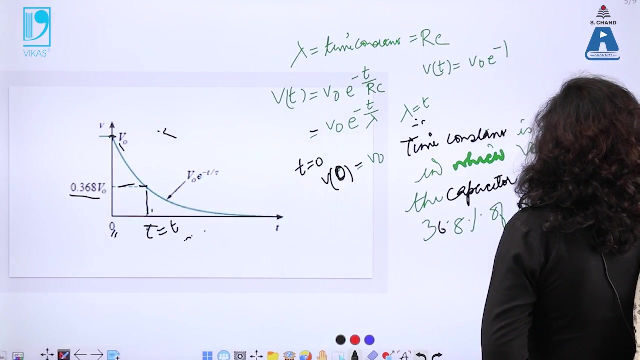 Definition says that time constant is that time in which voltage reduces to 36.8% of its initial value. So what is time constant? Time constant is that time in which voltage across the capacitor reduces to 36.8% of its initial value. 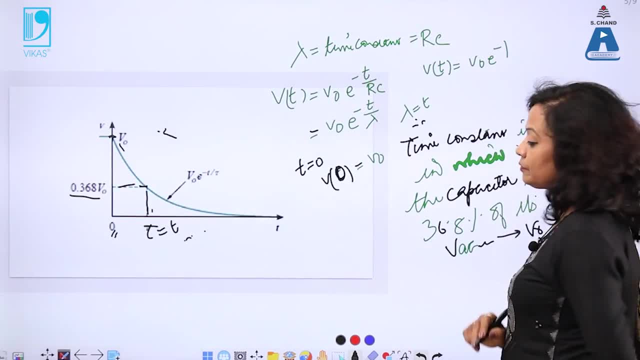 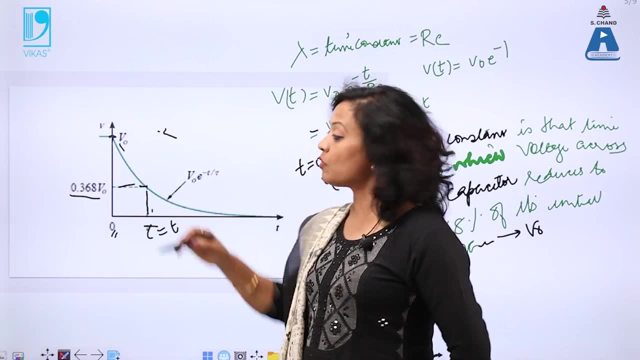 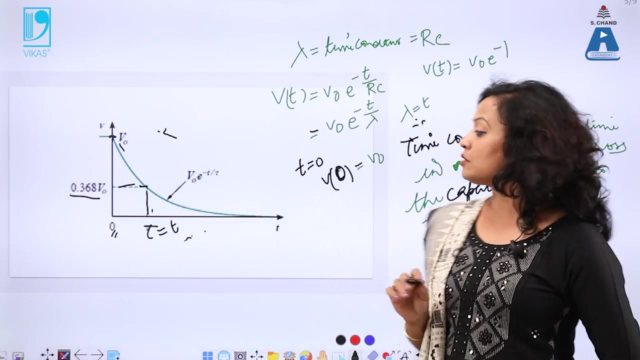 That is V0.. So this is source free, That is, capacitor is fully charged, There is no source, And capacitor is acting like a source And initially it is fully charged and finally discharged off. And time constant is that time in which that voltage reduces to 36.8% of its initial value, which is this. 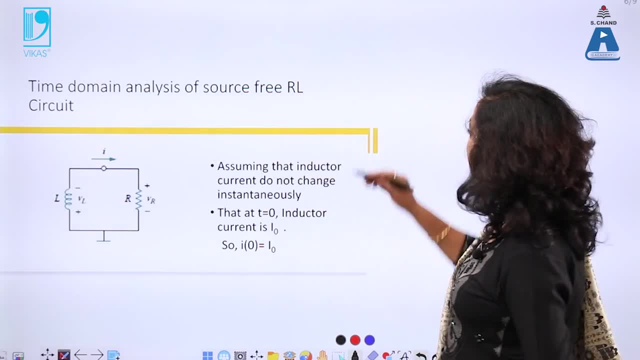 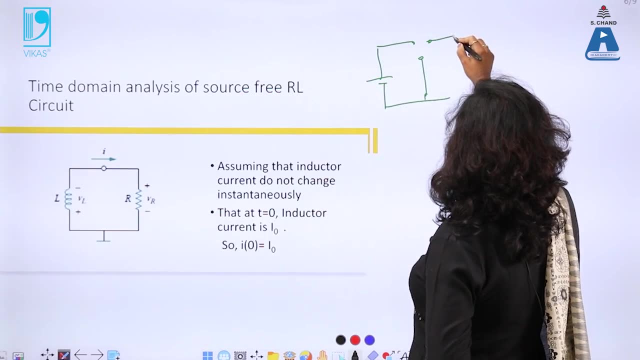 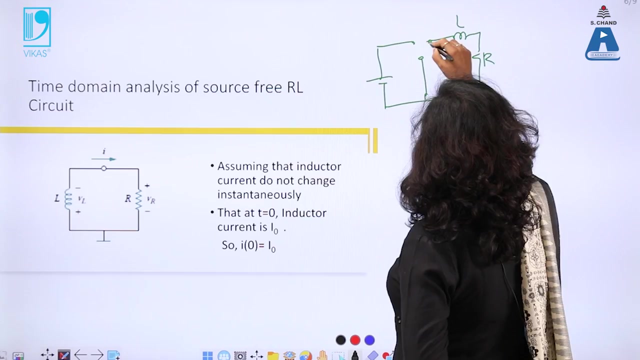 Then is time domain analysis of source: free RL circuit. Again, my circuit will be like this: Initially there will be two way switch. This is called as two way switch. I have inductor, I have resistor, So this is L and R and this is two way switch. 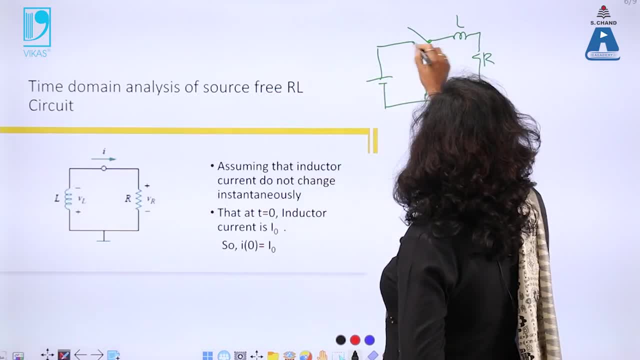 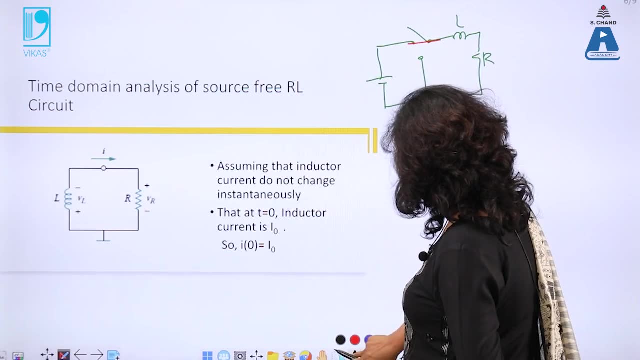 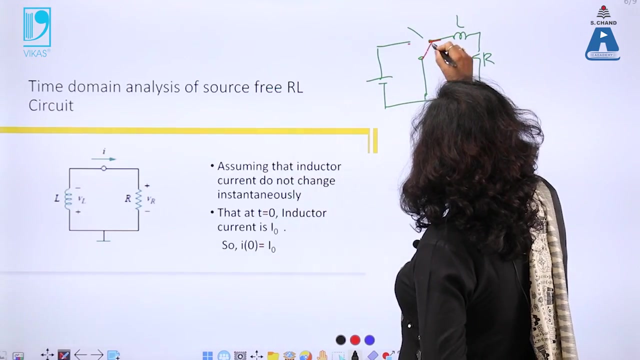 So initially, my switch is connected to this point, So there is energy stored in inductor. Now, as soon as I, as soon as, let me rub it. Yeah, So after some time, let I connect to this point. Now this is called as source free. 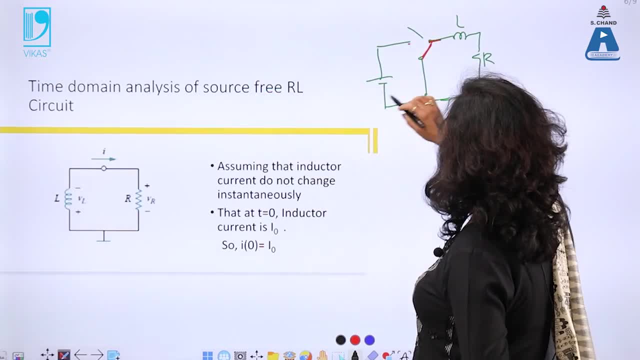 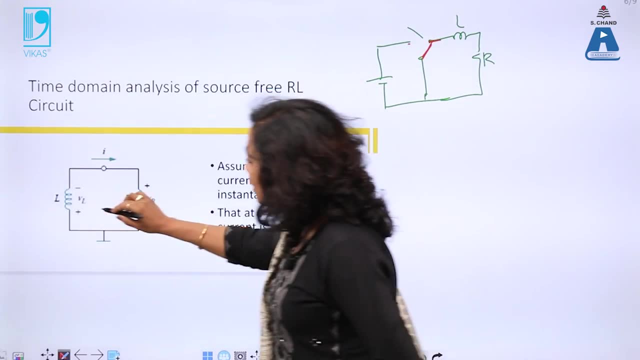 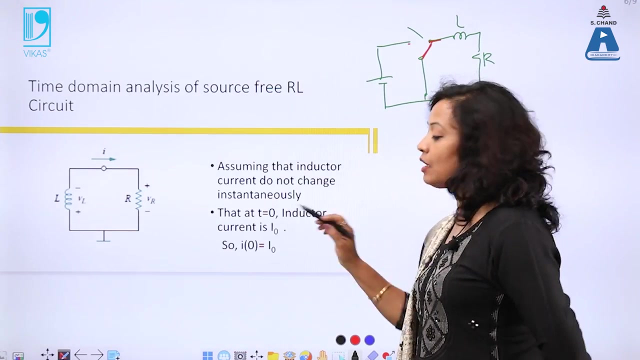 Source free, RL Source free circuit, because now there is no voltage source And the energy stored will be circulated in this circuit And finally it dies off. So let VL is the voltage across inductor And VR is the voltage across resistance. So at T is equal to zero inductor current, is I knot? 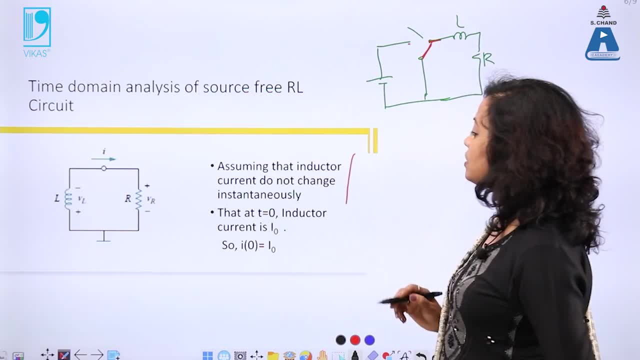 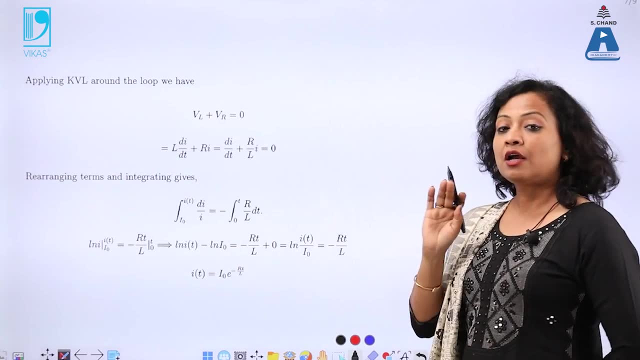 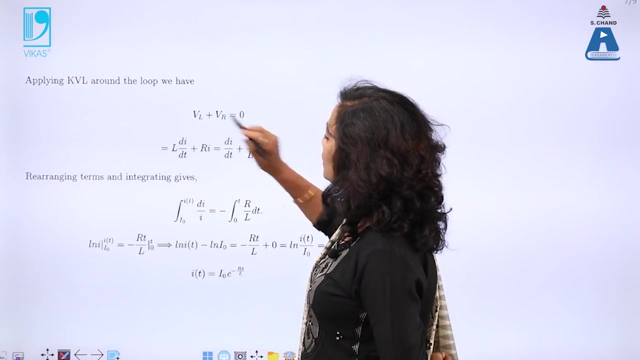 And we also say that inductor current do not change instantly. So that means whenever we switch the the switch, we change the switch. At that point of time time inductor current will not change, which will remain same. so if i apply kvl voltage across, 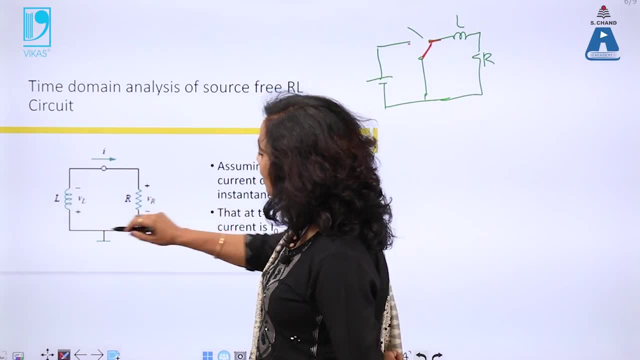 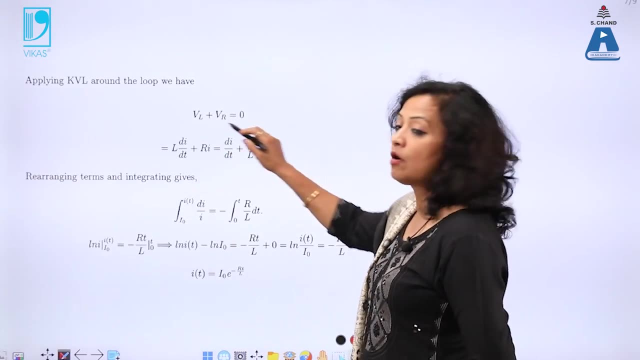 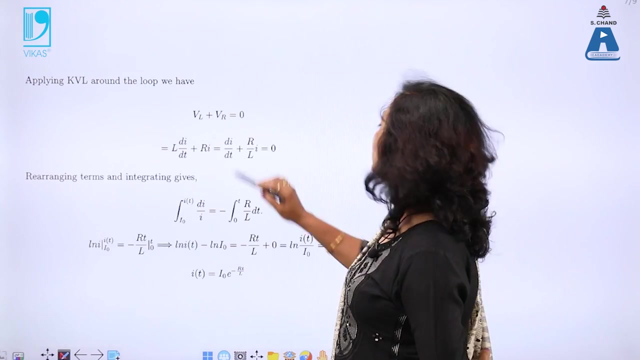 inductor. let me show you again. if i apply kvl, so as per kvl, voltage across inductor and voltage across in the resistance will be equal to zero, total voltage drop will be equal to zero. so vl is equal to ldi by dt, vr is equal to ir. so, reshuffling this, let r comes to this side i am. 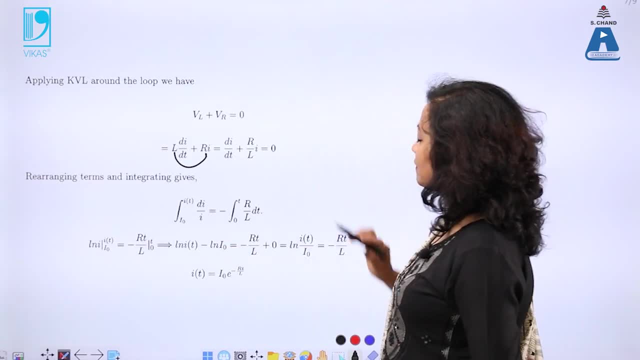 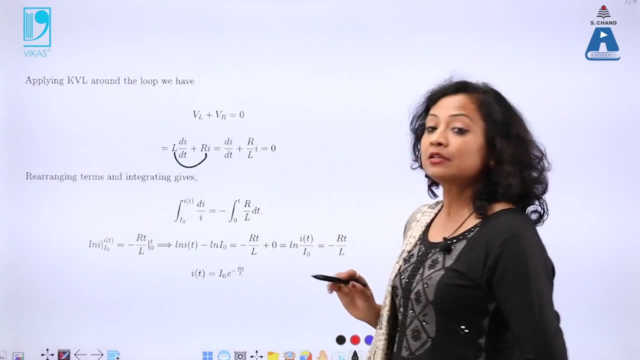 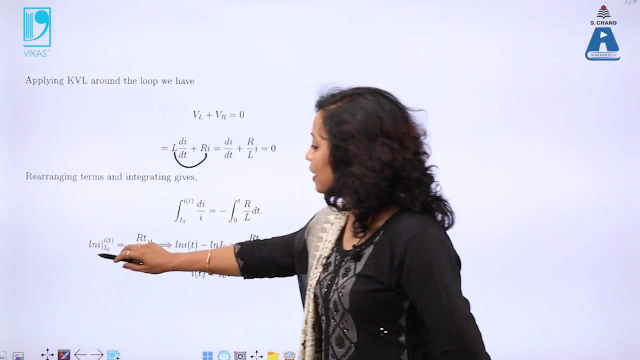 getting this, then di by di and then rest of the circuit, integrate from i not to it, i not is the initial current, which is the maximum current and it is a current at any instant of time is equal to zero, to t time second. and i, if i integrate, i am getting ln of i limits, i not to it and r by rt. 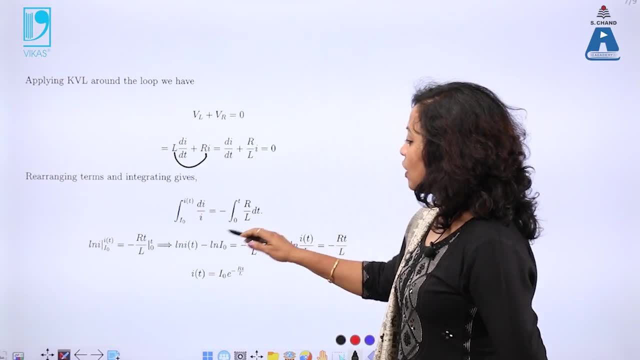 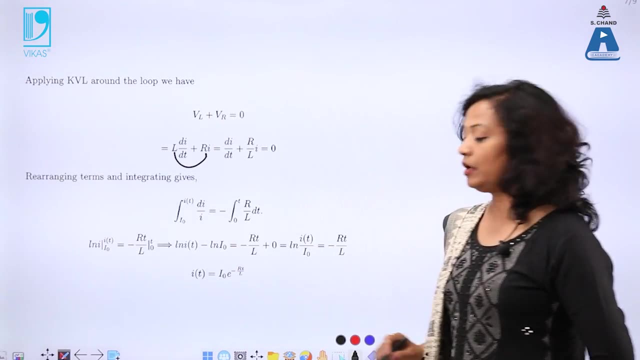 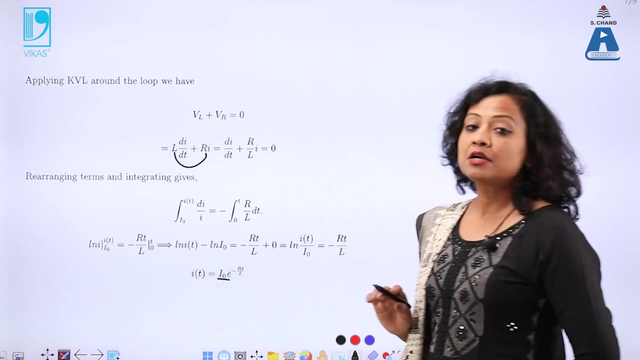 by l zero to t time. so if i solve it, ln of it divide by i not is equal to minus rt by l, or it is equal to i not e power minus rt by l. where i not is initial current at t is equal to zero. r and l is my circuit element and t is any instant of time at which we wish to see the. 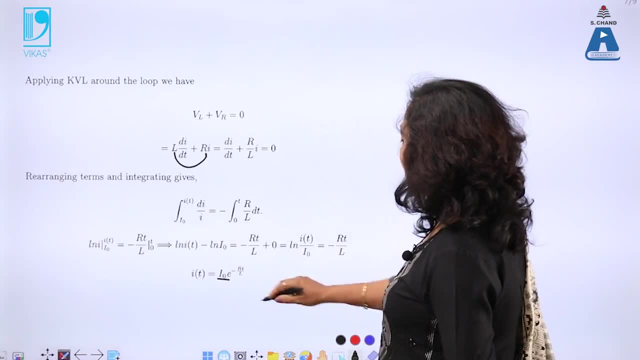 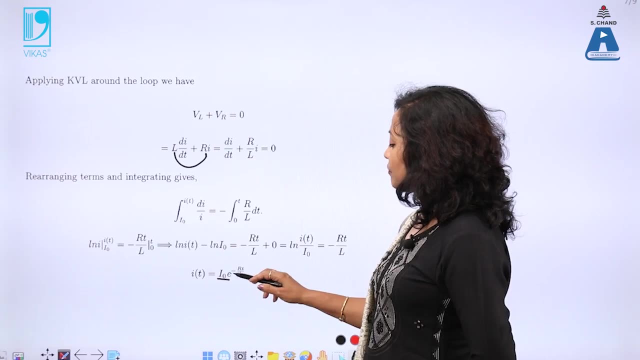 current. so we can see that. let me go back. so my final equation is: it is equal to i, not e, power minus rt by l. so initially, at t is equal to zero, i get some value of current, which is i not, and at t is equal to infinity, my current will. 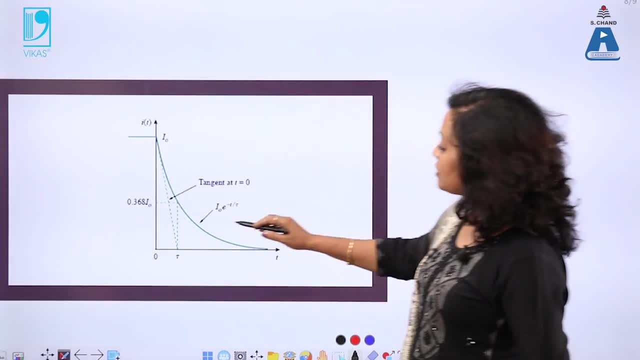 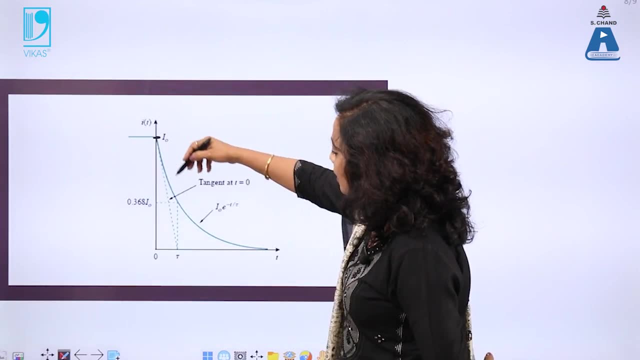 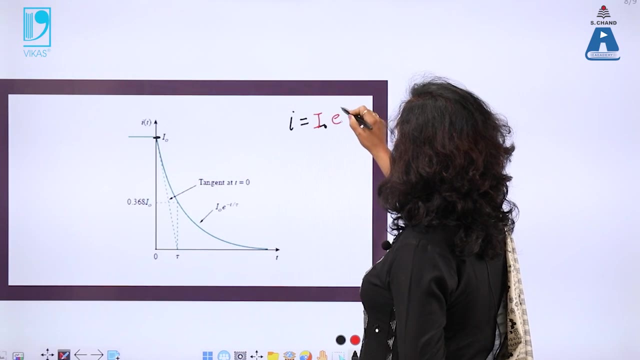 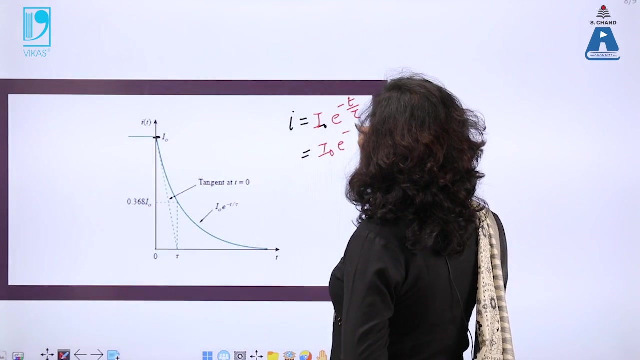 reduce to zero because there is no source. so you can see from this graph: initially, when t is equal to zero, my current is maximum, equal to i, not, and as t increases, it reduces to zero. so i is equal to i, not e power minus t by tau. or this is i, not e power minus rt by l. so you can see that lambda. 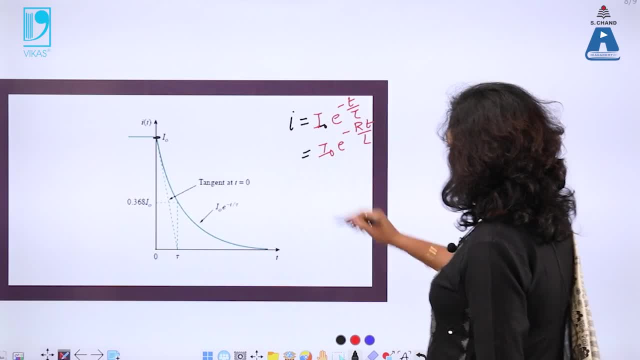 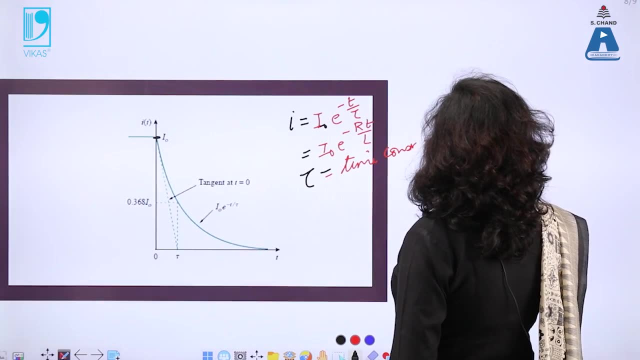 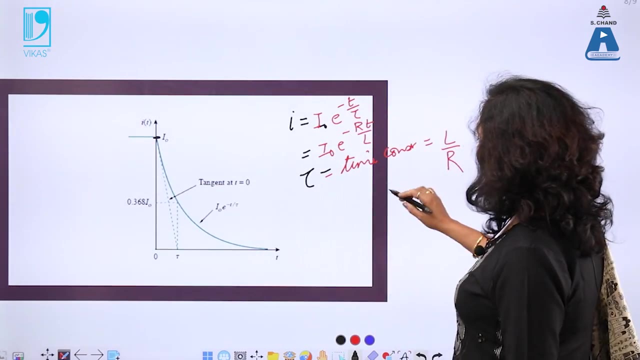 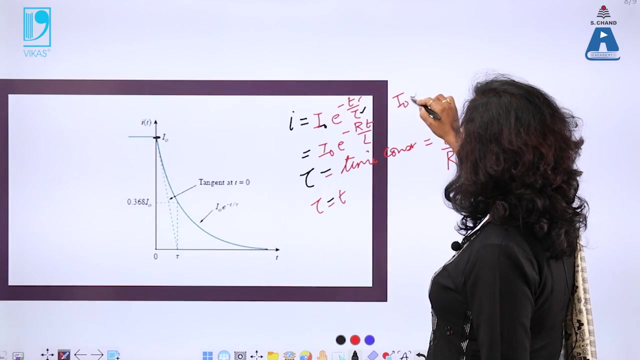 or you can say: not, lambda, this tau is equal to time. constant is equal to l by r. so based on value of l and r, i can define my time constant where, if i put tau is equal to t, tau is equal to t, i will get i, not e power minus one. and if i put the value of this exponential power minus, 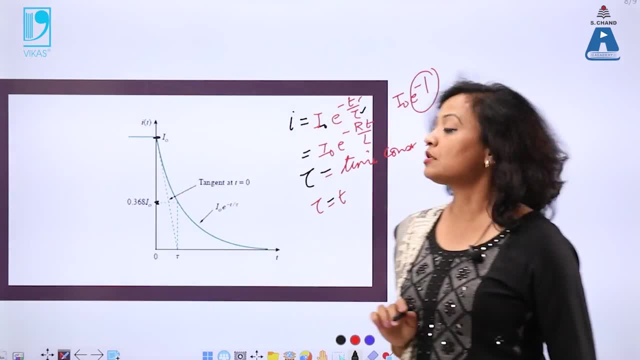 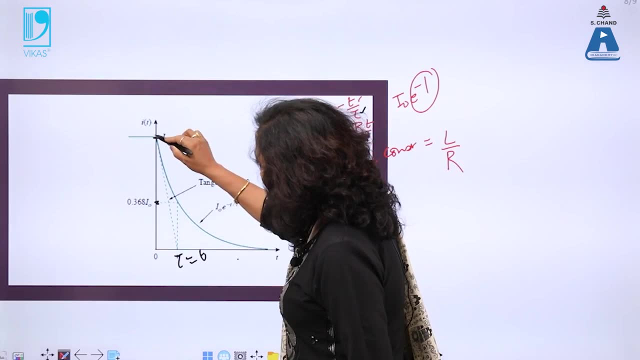 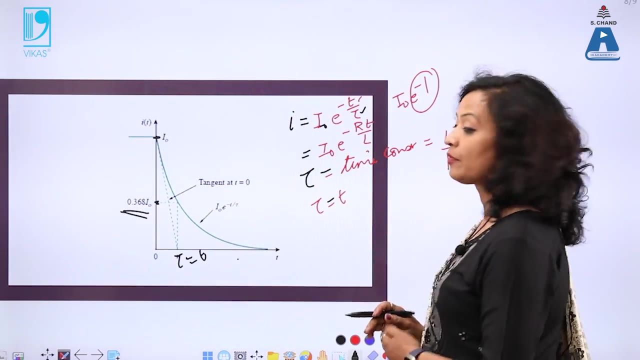 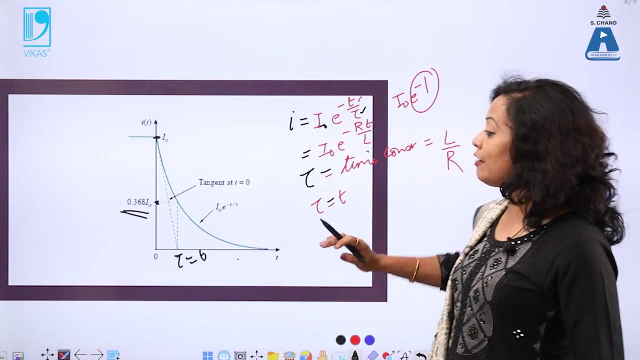 one, i will see that this comes to be 0.368 of i, not so time constant. this is tau. is that time in which my current initial current i not reduces to 36.8 percent of its initial value? this give me how, in how much time, my this current is going to reduce to zero. so that give me whenever i switch. 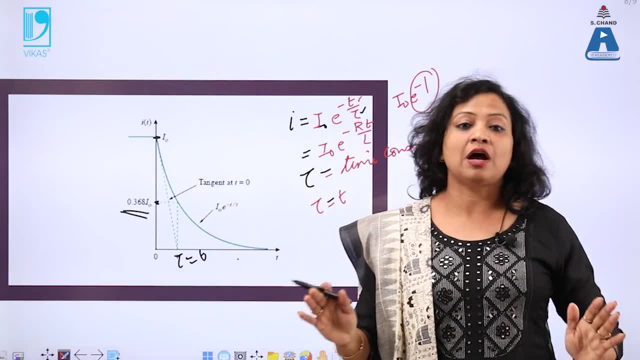 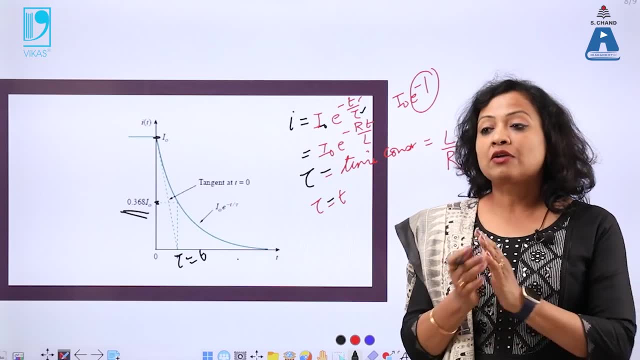 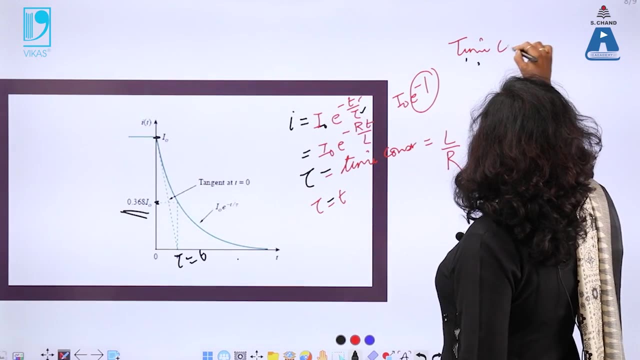 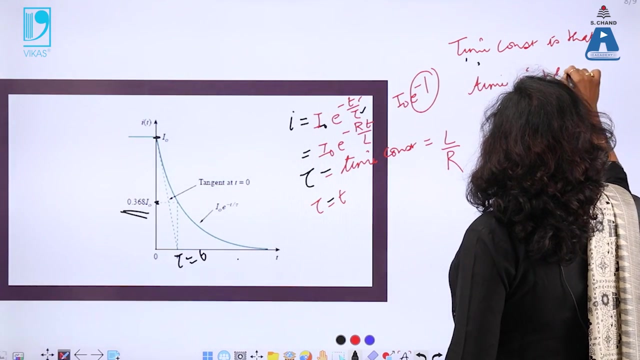 off my supply. that gives me what is the total diode of time in which my transient current is reducing. the shortest the time, the better is my system, because the transient time gives me slow response, so i can define that time constant: is that time in which the transient current 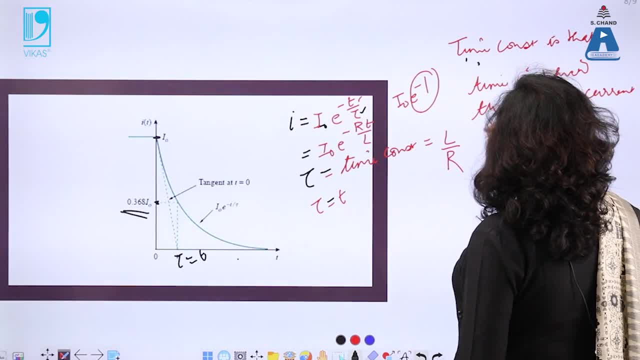 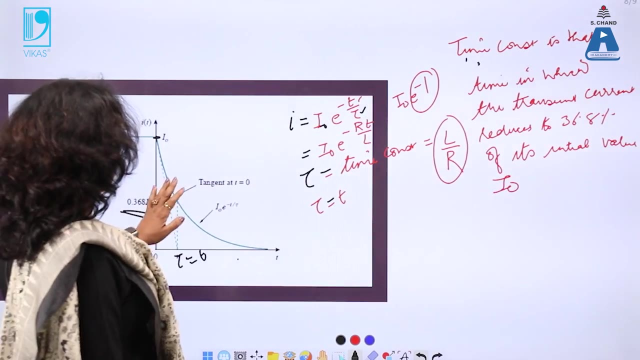 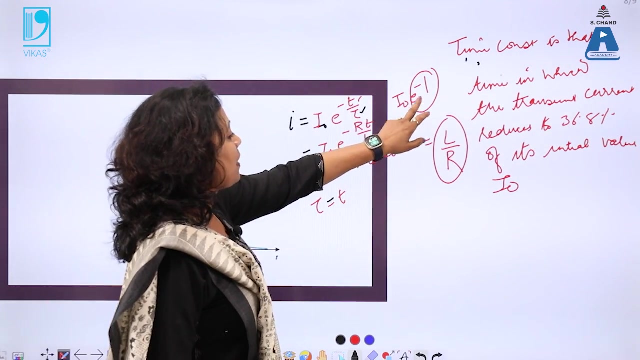 reduces to 36.8% of its initial value, I0.. So from this graph we can see that if I put, tau is equal to t, so I am getting I0 is e power minus 1.. So if I put the value of exponential minus 1,, 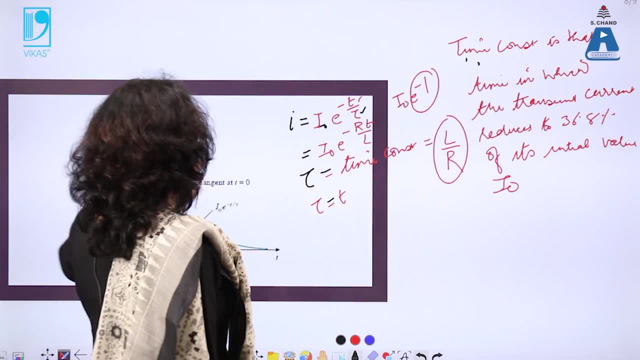 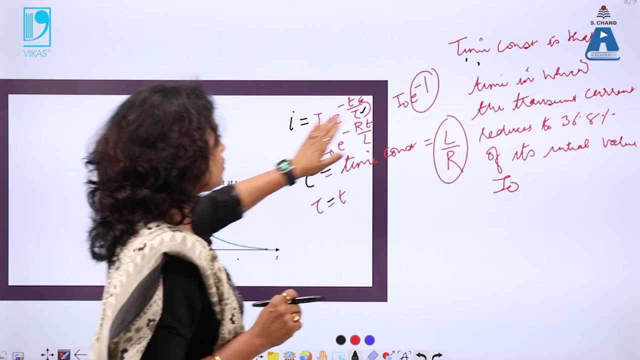 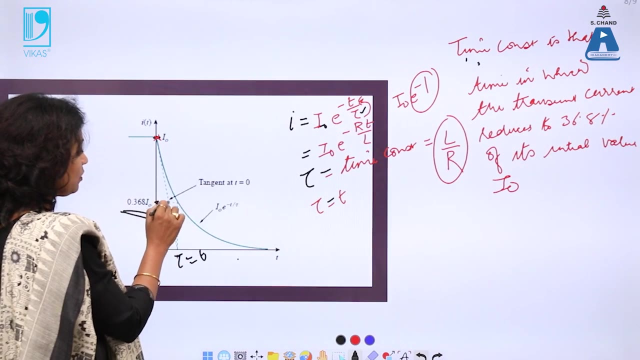 I will get 0.368 of I0.. So time constant is that time in which my current at any instant reduces to 36.8% of its initial value. That means initially it is there. So when I put, t is equal to tau. 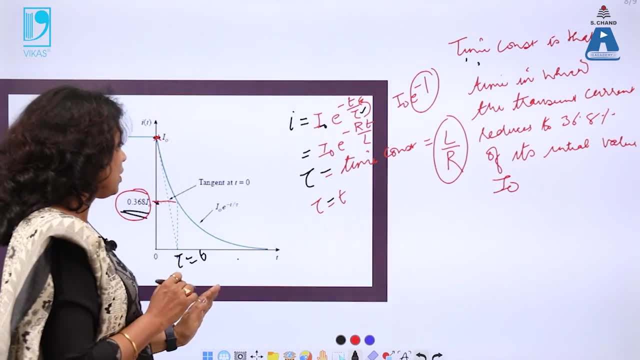 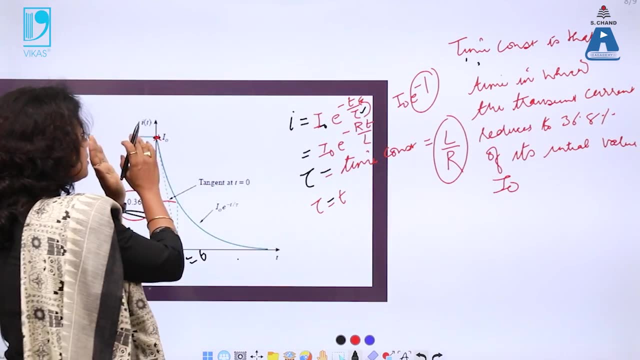 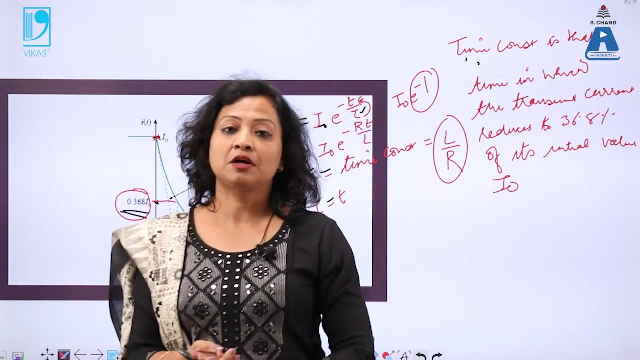 I am getting the value 36.8% of its initial value. So, based on my elements value Lnr, I can define my transient time in which my circuit current dies off. So shortest is the time, better is my system, because that will give me the response of my circuit. 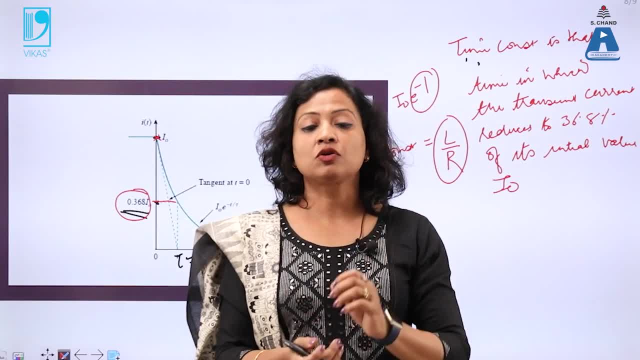 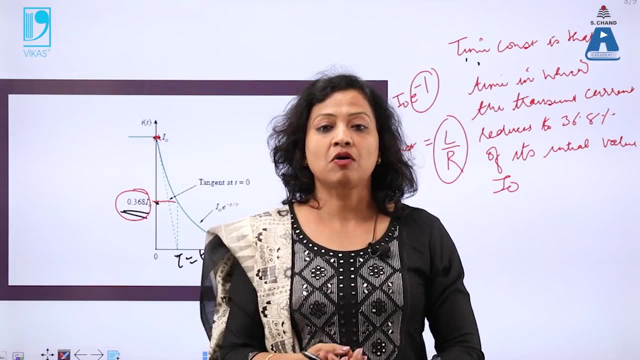 Response in the sense that I switch off my source and it should die off instantaneously, Though it do not die off instantaneously, but the lesser is the time, the better is my response or output. So this is all about time. response of RC and RL circuit.